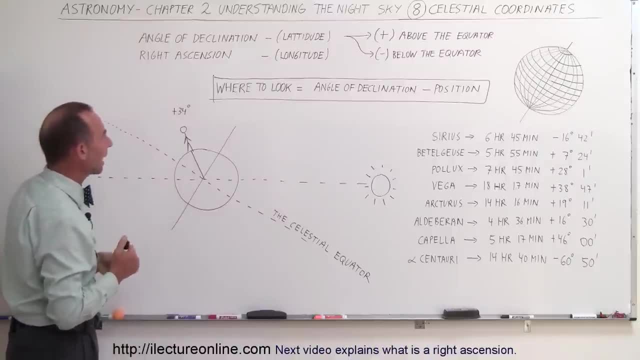 a negative angle for the angle of declination. So I have indicated that right there. So that's it. So now, of course, we're going to be observing things from some position on the Earth. I happen to live very near, 34 degrees north of the equator, near Los Angeles. 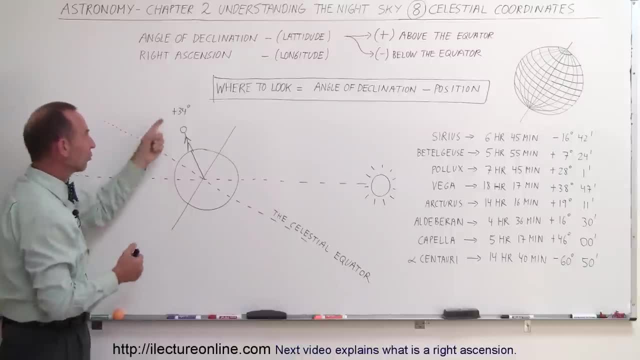 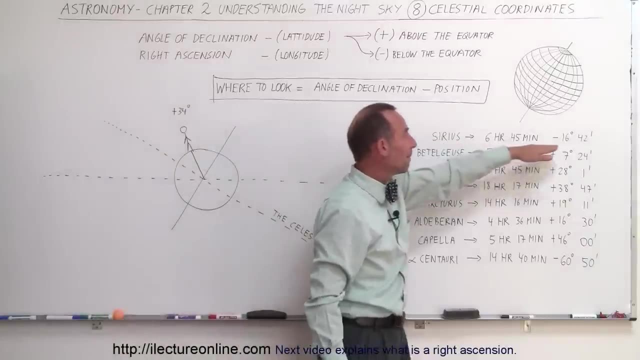 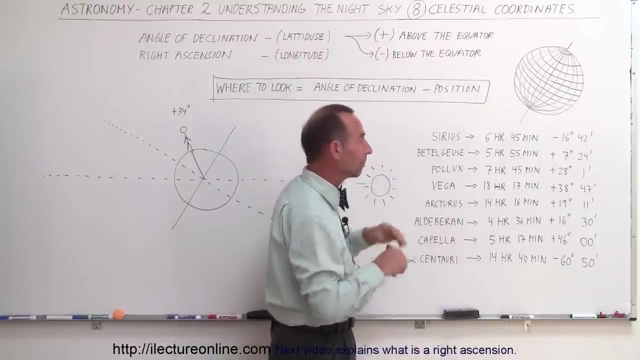 and so therefore, the angle of declination from my position is 34 degrees north of the equator. So now when we go over here, notice Sirius is at a position minus 16 degrees. That means it's actually in the southern portion of the celestial sphere, below the equator line. 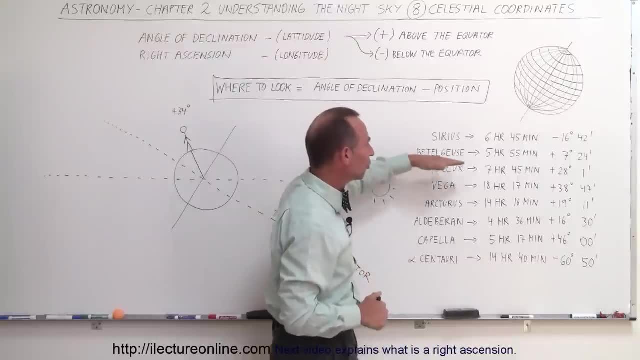 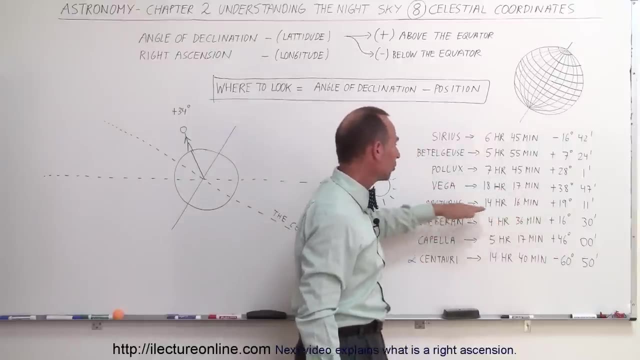 below the plane of the equator. The celestial equator: Betelgeuse is 7 degrees above. Pollux is 28 degrees above Vega: 38 degrees. Arcturus: 19 degrees. Aldebaran: 16 degrees. 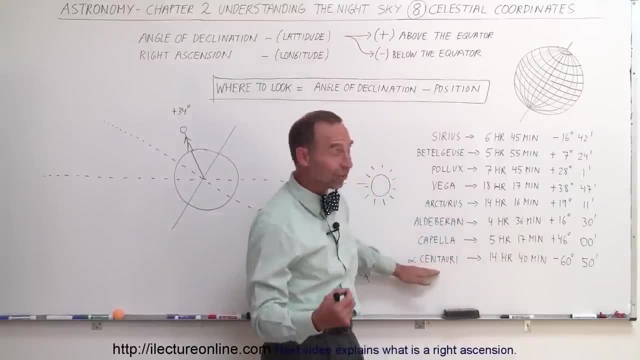 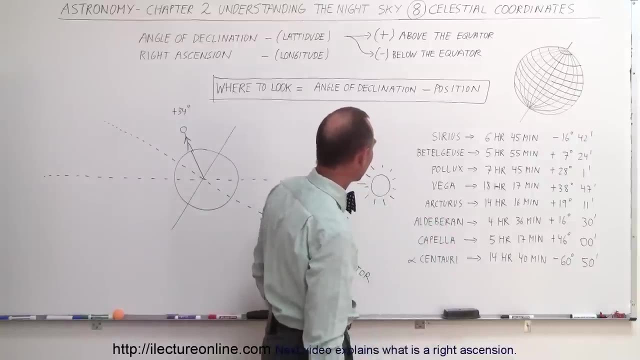 Capella, 46 degrees, And Alpha Centauri, the brightest star in the sky, which, no, it's not the brightest, it's the closest. The brightest is. where did I don't have it on here? Oh, yeah, there it is Sirius. 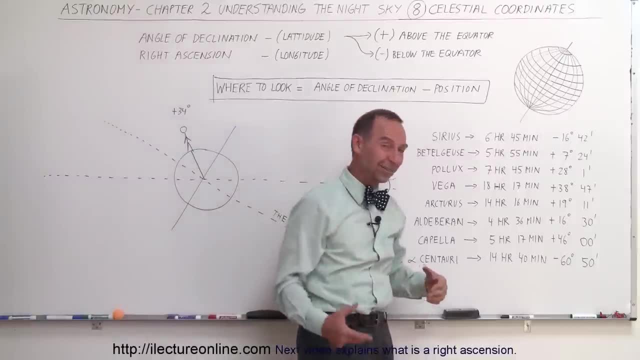 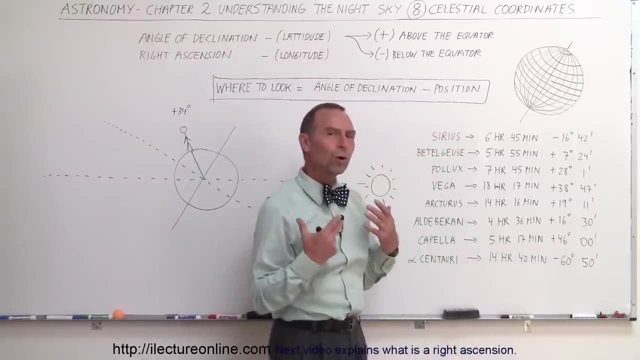 The brightest star is Sirius. Alpha Centauri is one of the brightest- About the fourth brightest, but it is the closest. It's at minus 60 degrees. So where should we be looking? Of course, at different times of the night and at different times of the year. 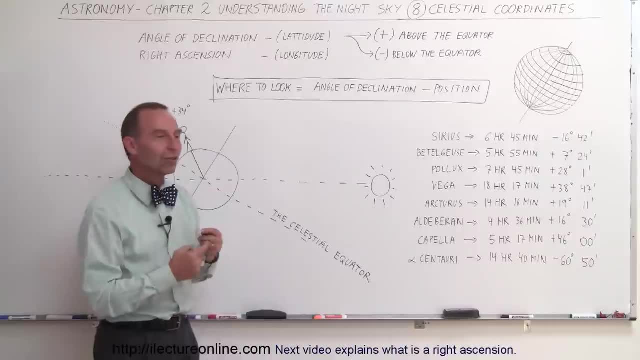 They're going to be in different positions relative to the rotation of the Earth and relative to the Earth revolving around the Sun, But at some point, once every 24 hours, that star will pass through the meridian, through the line that goes from the North Pole to the South Pole. 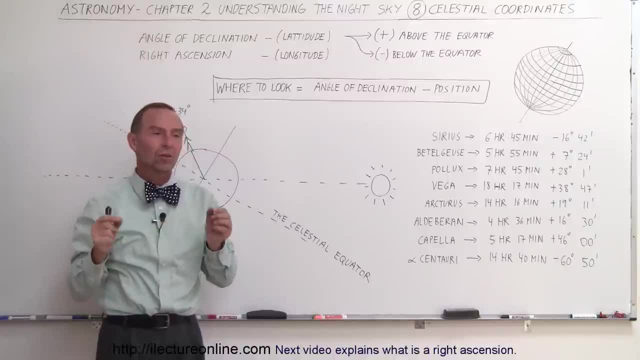 and through the point directly above our head which is called the zenith. So, once per 24 hours, any one of those stars, any constellation, will go through that meridian, And so if we're at the moment that it goes through the meridian, whatever it may happen to be, 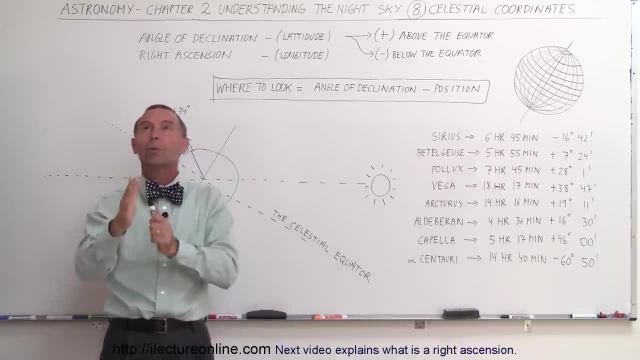 2 o'clock in the morning, 8 o'clock at night. whatever it may be, where will it be? Do I need to look directly upward? Do I need to look towards the horizon? Do I need to look in the other direction? 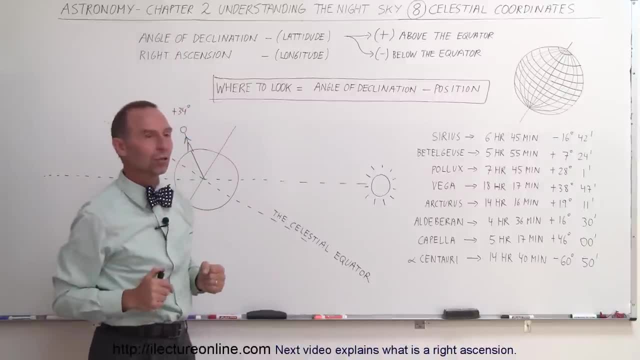 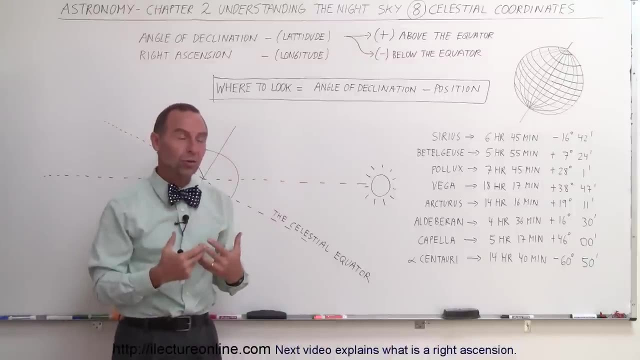 Where should I look? Well, that depends on the angle of declination. Now, if the star, or whatever it is, depends on the angle of declination, Well, that depends on the angle of declination. the star, or the constellation, is at 34 degrees north, so plus 34 degrees. 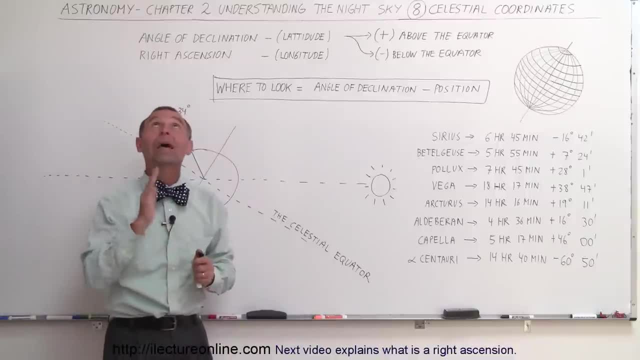 since I'm already at 34 degrees north of the equator. I would then have to look straight up. But where should I look if it's greater than 34 degrees? Where should I look if it's less than 34 degrees? Well, if it's greater than 34 degrees, that means it's closer to the North Pole than I am. 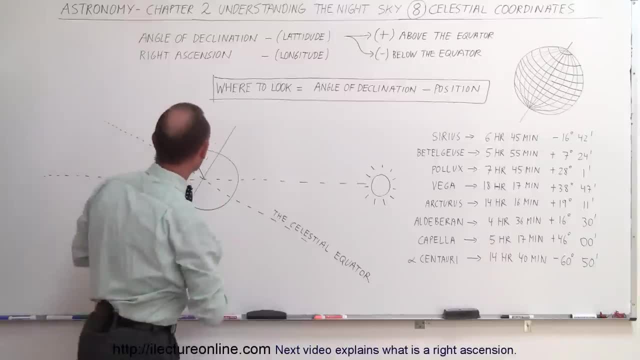 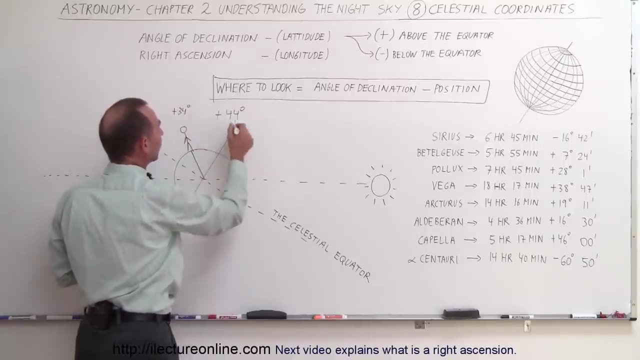 so I have to look in a northerly direction. For example, if I'm at 34 degrees north and another star is at 44 degrees north plus 44 degrees, that means it'll be at some location over here at 44 degrees north of the equator. 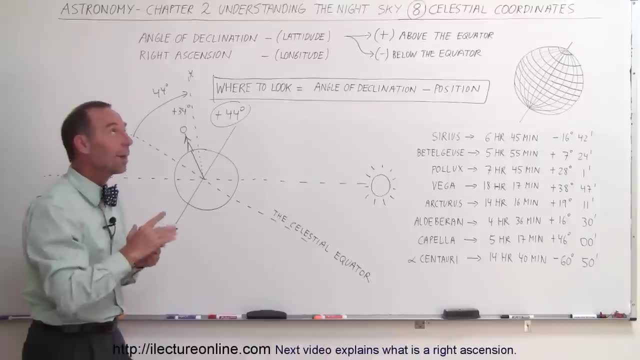 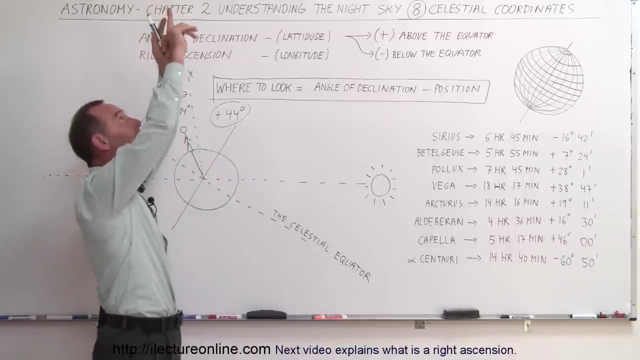 which means it's 10 degrees further north than where I am at. so instead of looking straight up at the zenith, I need to look at a position 10 degrees away from the zenith. Remember that the zenith is straight up in any direction. 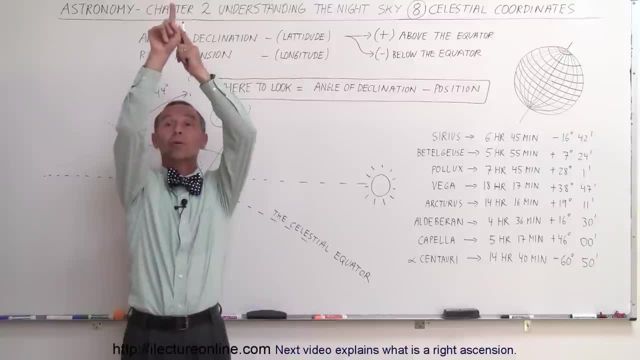 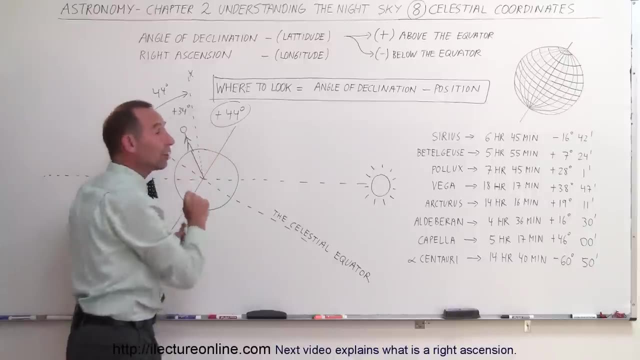 down to the horizon, no matter which I'm looking is an angle from 0 to 90 degrees, an angle from 0 to 90 degrees, and so forth. So that means if it's at 44 degrees, it's 10 degrees away, 10 degrees closer to the north. 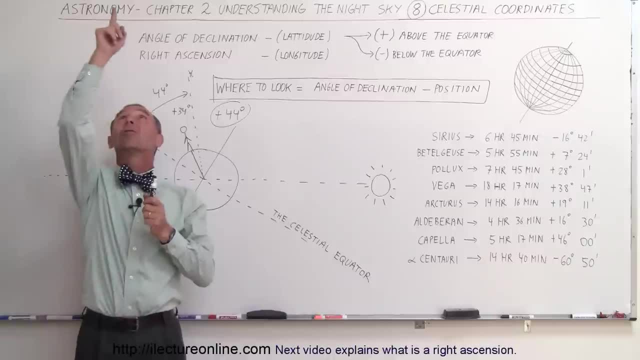 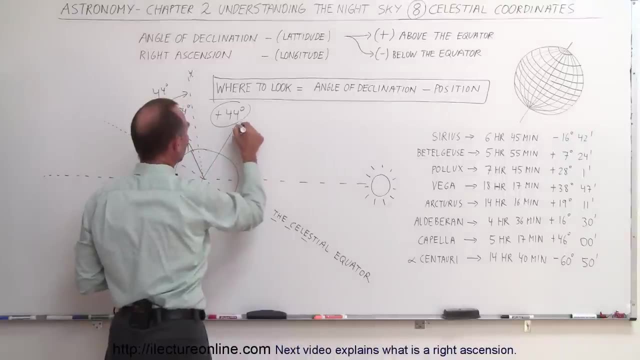 so I phase the north. for me, north is in that direction. straight up is the zenith. 10 degrees would be a 10 degree angle. I'll be looking for it over there If the star is at the North Pole, which is at 90 degrees, for example, Polaris. 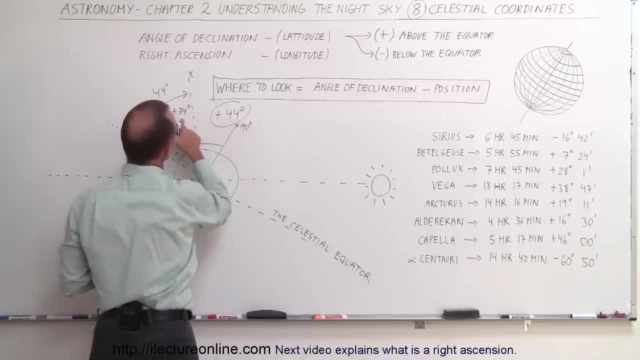 well, that is at an angle of 90 minus 34, which is 56? 56 degrees. So if I add 56 to this I get 90, so for me to find Polaris, the North Star, I have to look at an angle of 56 degrees away from the zenith. 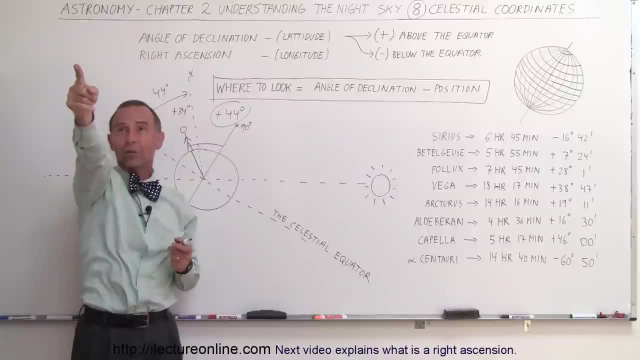 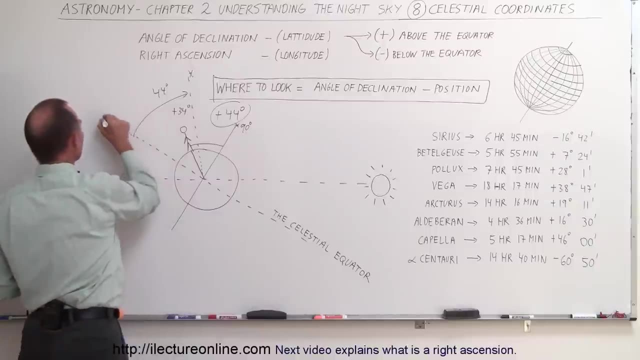 The zenith is directly above me 56 degrees. we'll put it right over there. that's where I should be looking for the North Star. What about for a star directly above the equator? Where should I be looking if the star is right here? 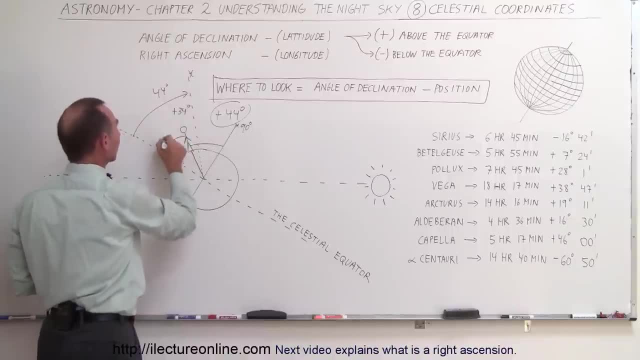 directly above the equator. Well, that's south of me. how many degrees? Well, that's 34 degrees south of me. so I have to turn around. south for me is in that direction. the zenith is straight up, and then I would look at an angle: 34 degrees away from directly north. 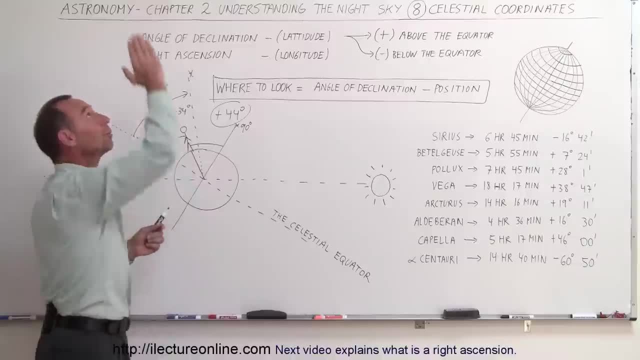 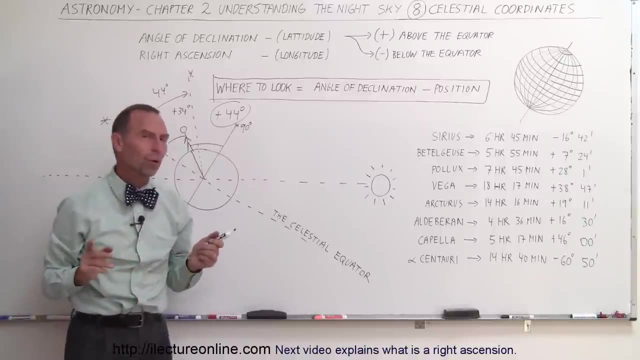 remember, 34 degrees is a little bit more than one third from directly north to the horizon. so I'll look at about an angle, about this big and be looking for it in that direction, But of course that would only be at one time. 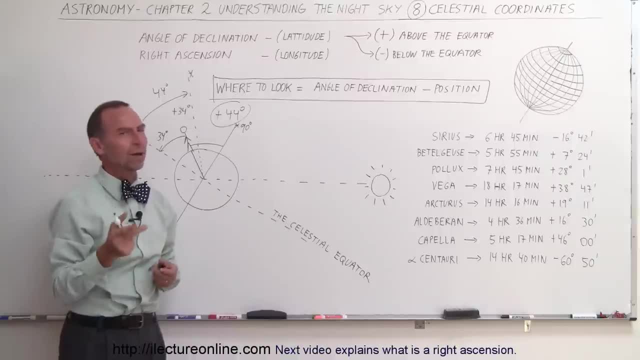 either during the daytime or the nighttime and of course, if it happens in the daytime I'm out of luck. if it happens at nighttime, I have to wait until it appears near the meridian. I look for it in that angle. At the next video we'll figure out how to look for it at different times of night. 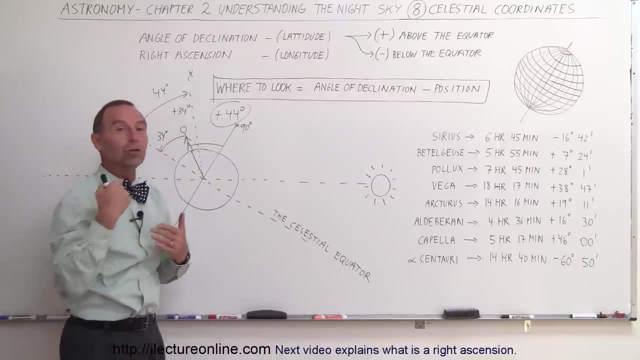 depending upon where it will be relative to the longitude, not the latitude, Of course. longitude in the celestial sphere is called the right ascension, and we'll tell you about how to look for it there, But a general approach as to how to look for stars. 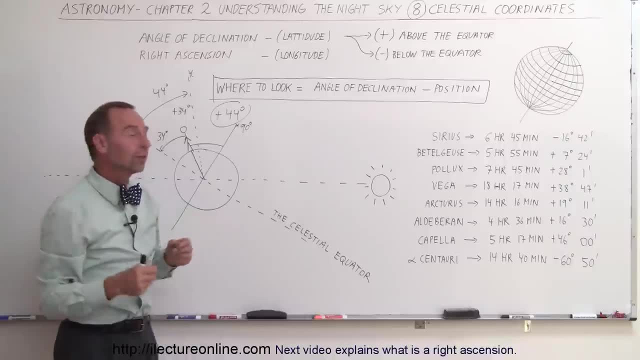 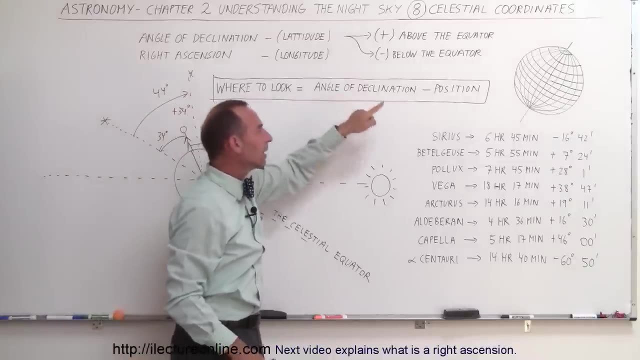 as far as where the position will be: relative to the equator, relative to the North Pole, relative to the South Pole. we use this principle right here. Where to look? We look for the angle of declination, which is right here. 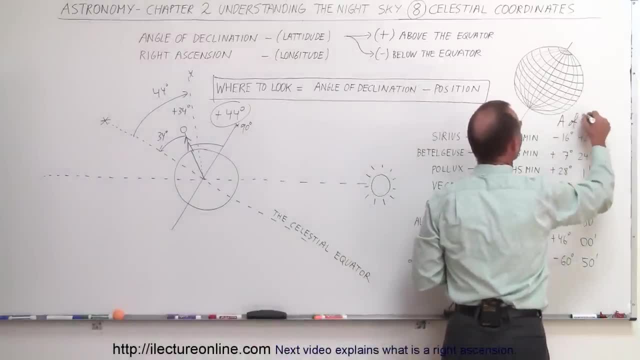 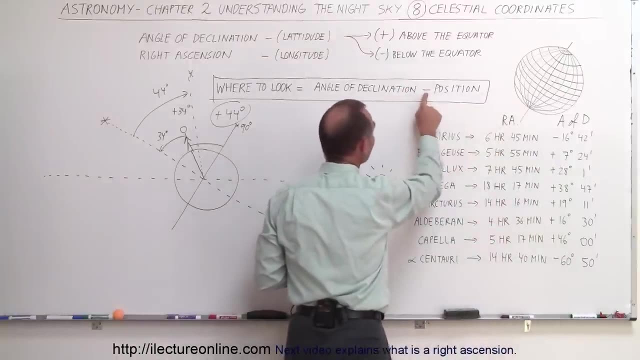 this is the angle of declination. so, angle of declination, this is right ascension, as we call it, and so we look for the angle of declination and we subtract from that the position of where we're at, and we should be able to look for that star there. 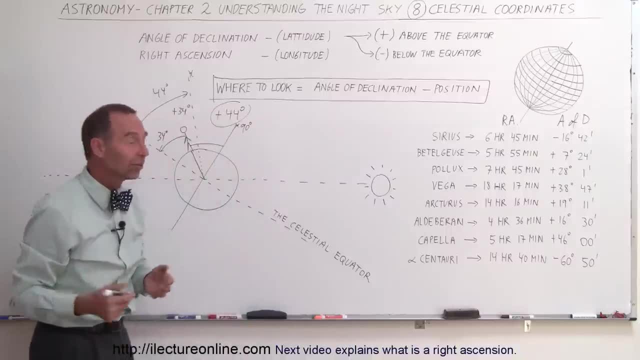 So let's try a couple. let's look for Sirius, the brightest star in the sky. so where to look? We take the angle of declination, which is minus 16 degrees 42 minutes. but I'll just go ahead and round it off. 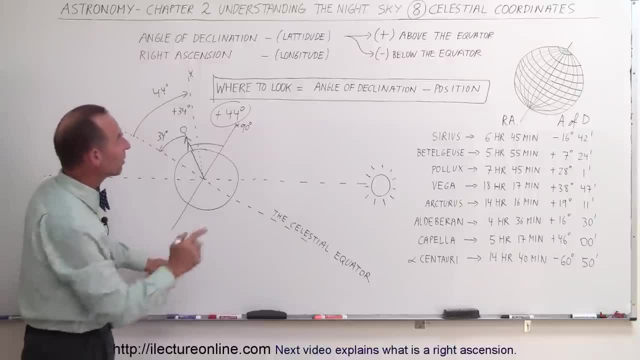 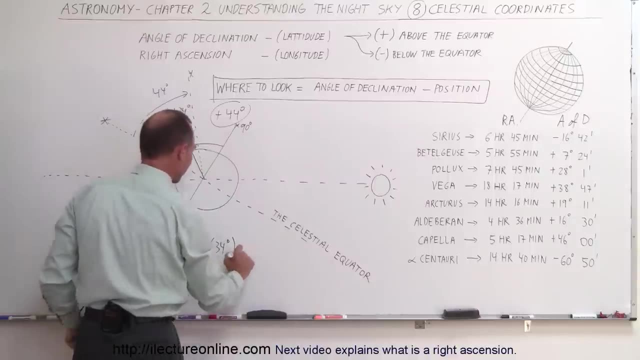 or just take the minutes only. I should say the degrees only. so minus 16 degrees minus the position I'm at, and I'm at 34 degrees. so minus 16 minus 34 is equal to minus 50 degrees. Now remember. 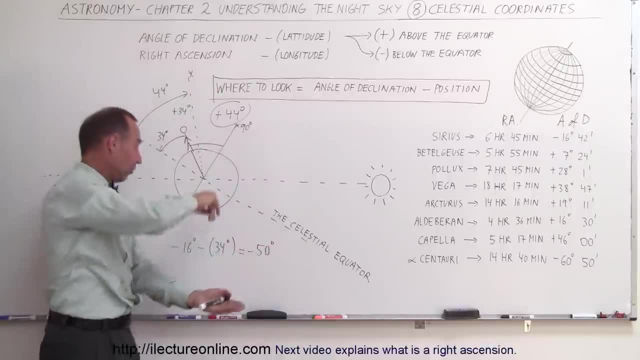 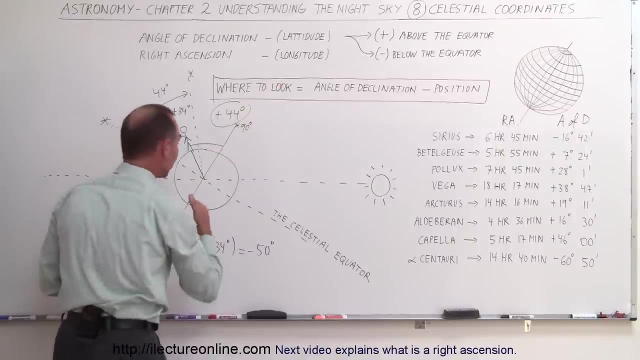 45 degrees is halfway between the zenith and the horizon, so 50 degrees is a little bit more, a little bit further down from the halfway point. Negative means I have to go look towards the south and 50 degrees below the point directly above me. 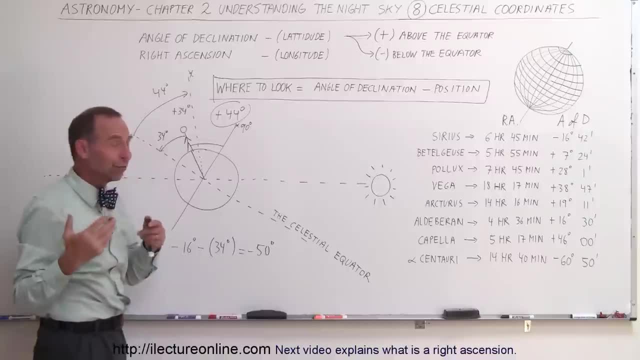 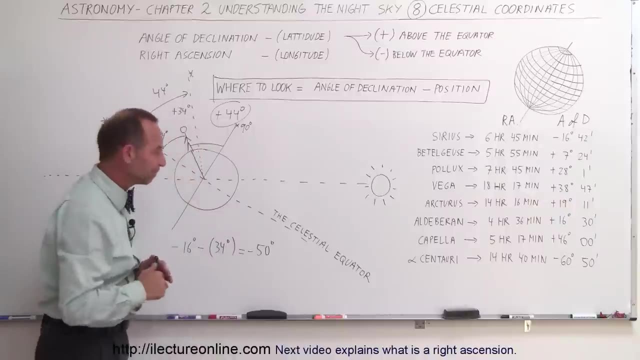 so in that direction, right there. So if I want to look for Sirius, I have to look towards the south at a 50 degree angle below the point directly above me, or 40 degrees up from the horizon, whichever way you want to look at it. 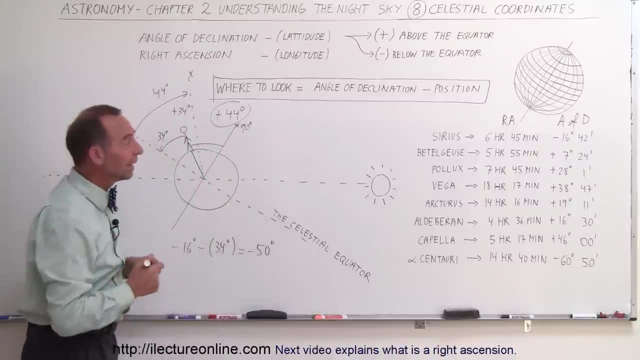 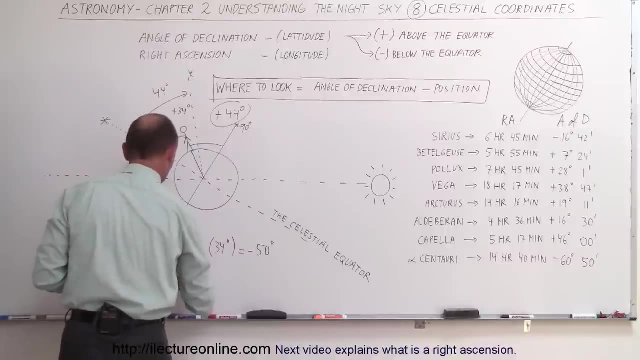 Okay, let's take the next one. Betelgeuse is that big red giant in the constellation of Orion and it's at 7 degrees above the equator. so I use my equation: plus 7 degrees, minus 34 degrees. 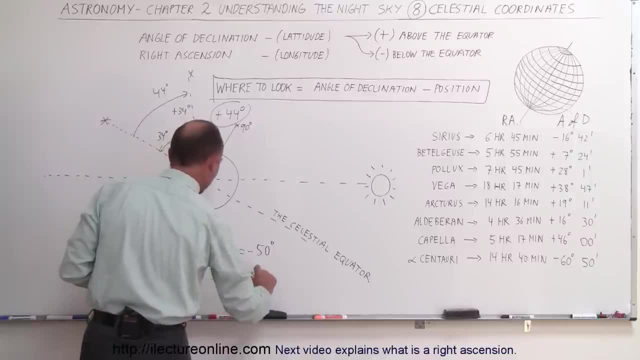 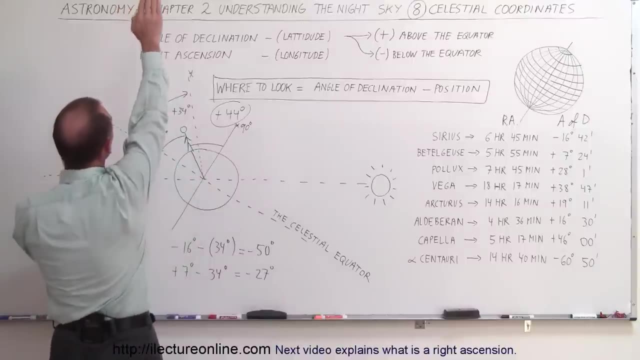 that's the location where I'm at- is equal to minus 27 degrees. So I'm looking for Betelgeuse at an angle of minus 27 degrees, so I look straight up, then I go 27 degrees this way, looking towards the south. 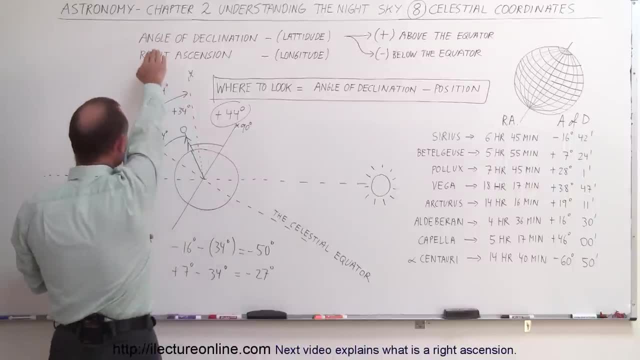 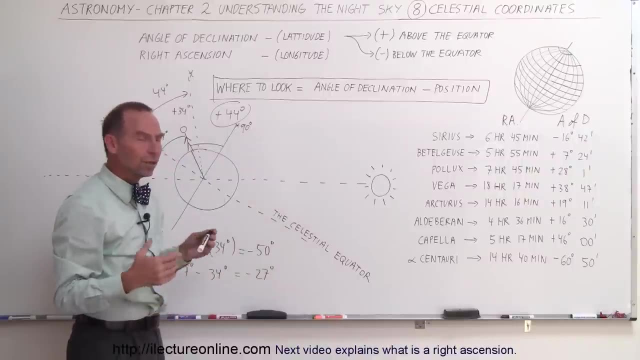 because it's negative. it's close to the equator, so I look 27 degrees away from the point directly above me. Let's try one more. How about Pollux? Pollux is one of the bright stars, probably the brightest star in Gemini. 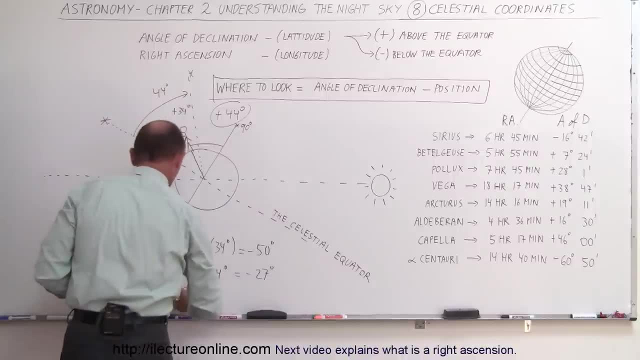 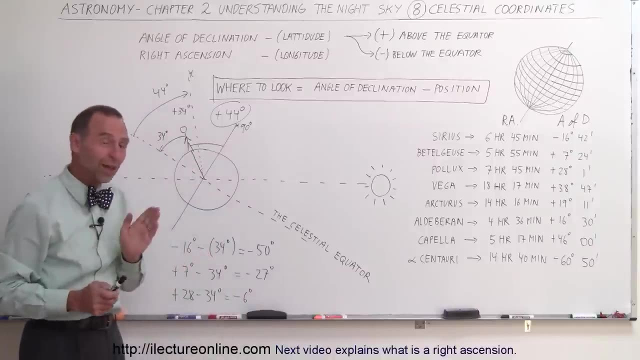 the twin and it's at 28 degrees. so I go plus 28, minus 34 degrees, which is minus 6 degrees. That's only 6 degrees towards the south from where I'm standing. 6 degrees, that's a very small angle. 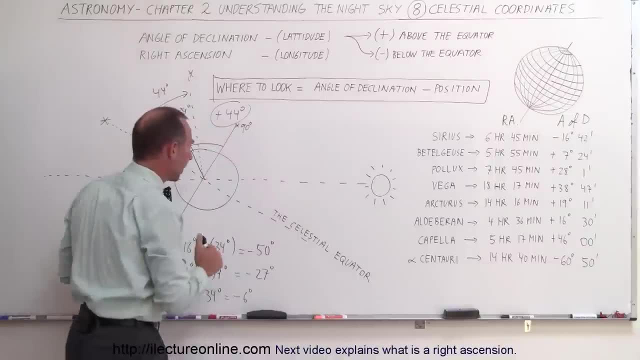 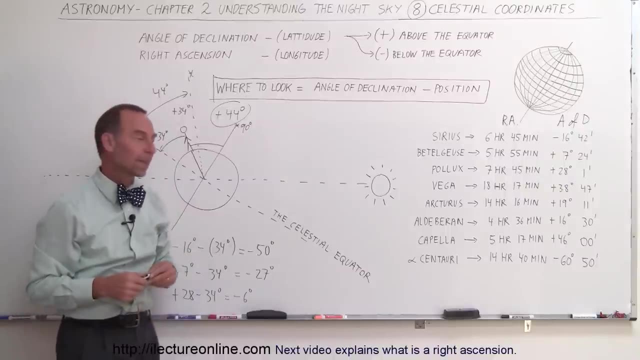 so Pollux will pass almost directly overhead if I'm looking at the night sky at the right time of the day, at night, and at the right time of the year. One more: How about Alpha Centauri? Well, it's at minus 60.. 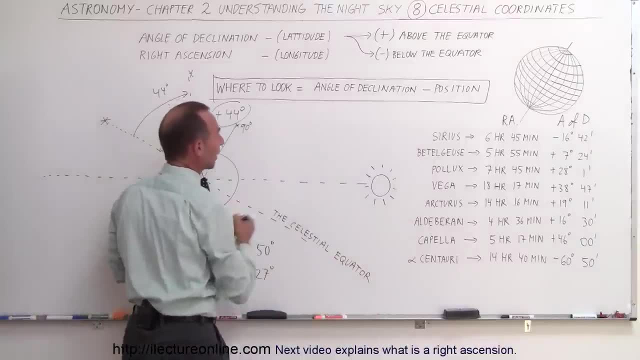 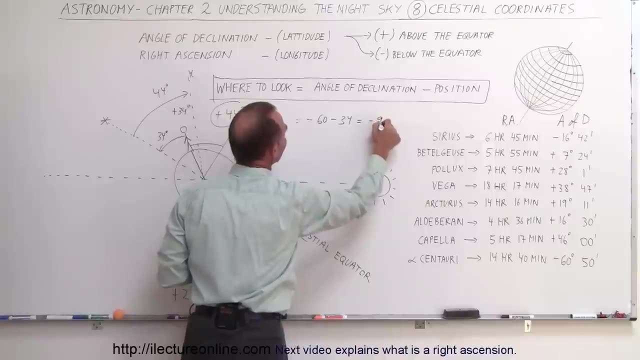 Wow. So I take my equation, so I take where to look. the angle of declination would be minus 60, and I subtract from that, my position is minus 34, which is minus 94. That's more than 90 degrees. 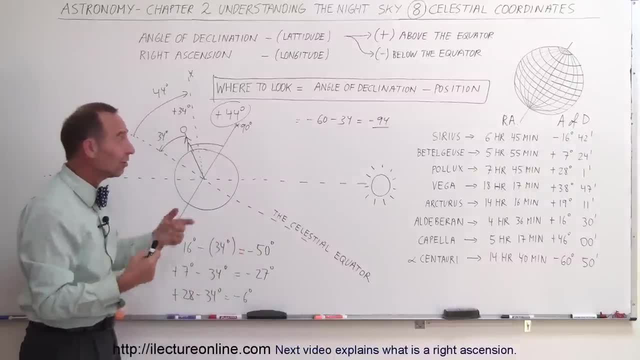 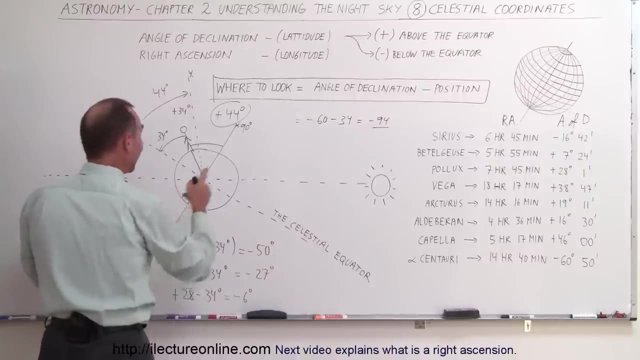 That's past the horizon. So from where I'm standing, near Los Angeles, if I want to see Alpha Centauri, I'm out of luck, because first of all it's minus, so I have to look towards the south. 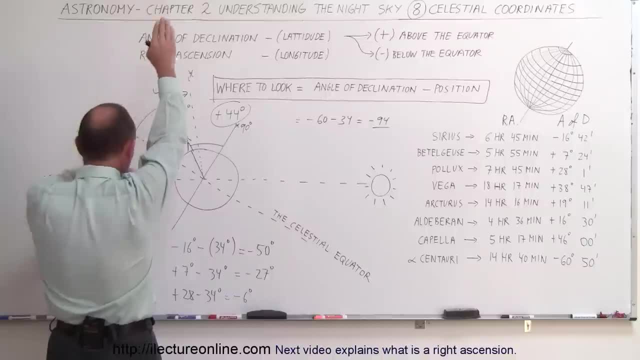 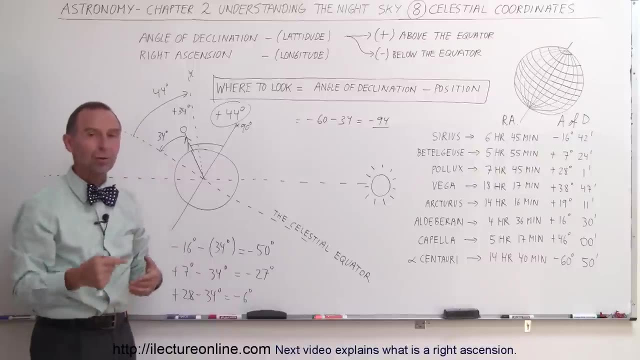 94 degrees. so the zenith is up there. 94 degrees puts it past the horizon. There's no way that I can see Alpha Centauri from where I'm standing. I'd have to travel south, maybe towards southern Mexico or towards South America. 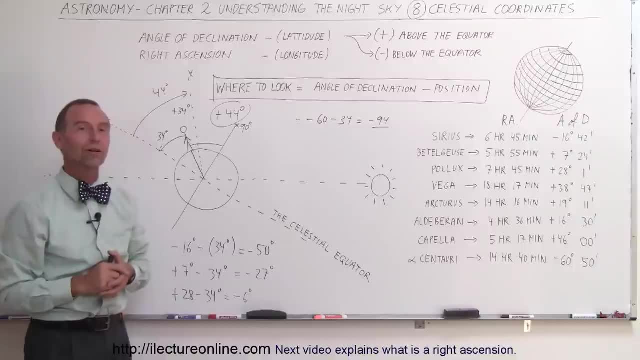 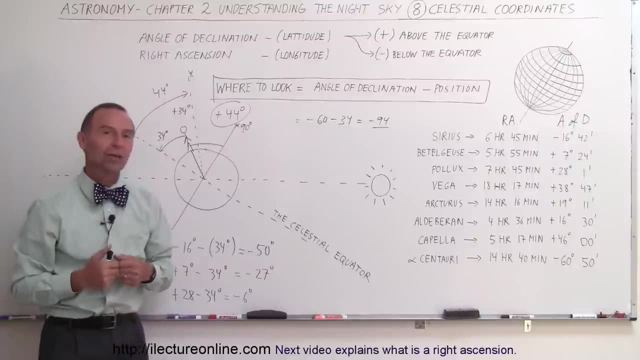 or the Panama Canal or something, before I can start looking for the star Alpha Centauri. So that's how we use the concept of angle of declination to find the stars. In the next video we'll attack the concept of right ascension.